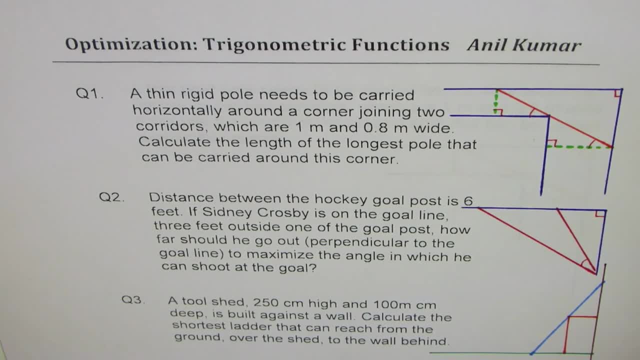 I'm Anil Kumar. Welcome to my series on trigonometric functions. Now we'll discuss three very important optimization questions based on trigonometric functions. I've given the diagrams with the questions also so that you can really understand and solve these questions on your own Take. 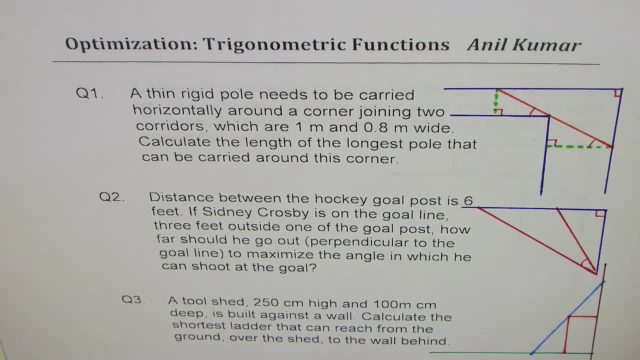 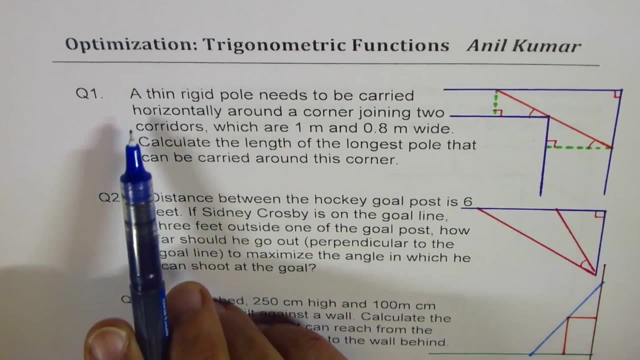 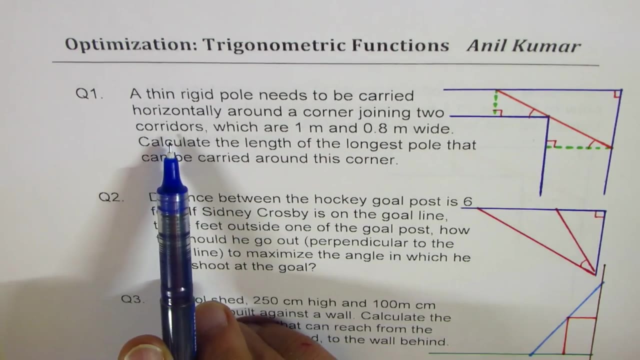 time to copy these questions, solve and then look into my suggestions. Now let's discuss Question number one. here is a thin, rigid pole needs to be carried horizontally around a corner joining two corridors which are one meter and 0.8 meter wide. Calculate the. 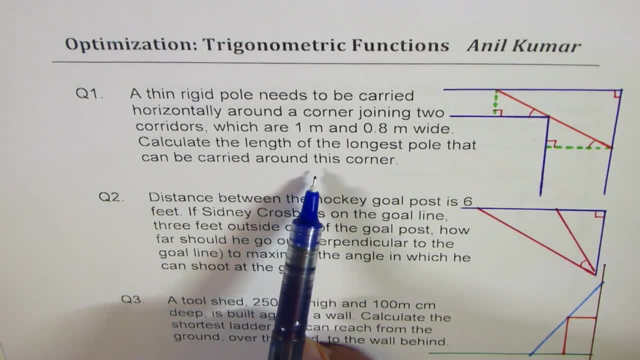 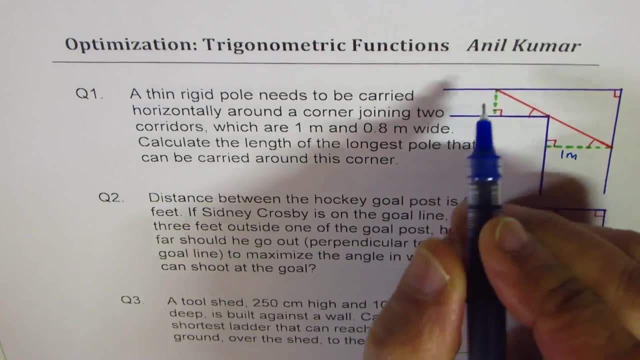 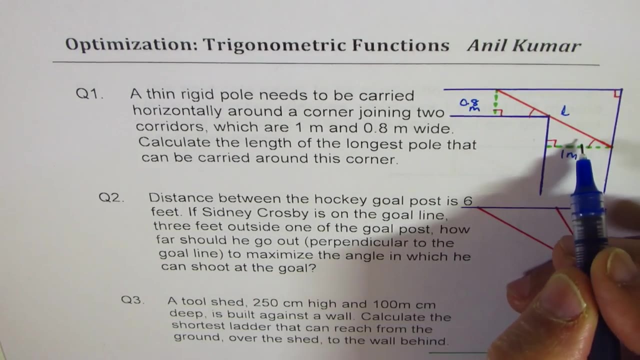 length of longest pole that can be carried around this corner. So we are given this corridor. One of them is one meter, the other one is 0.8 meters and that is the length of the pole, right? So if you say that this is angle theta that. 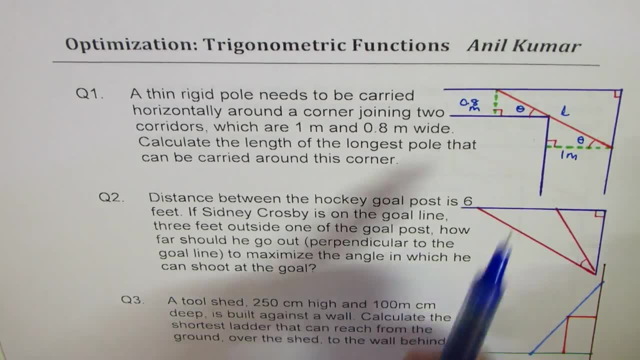 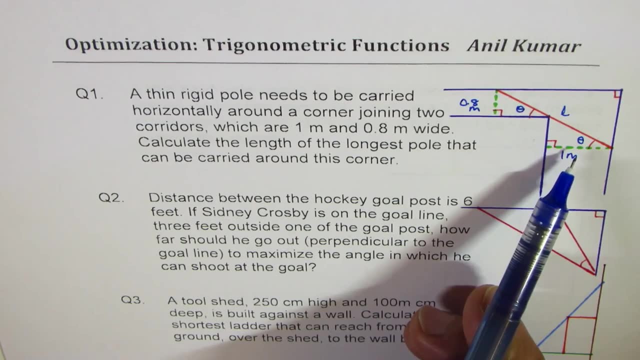 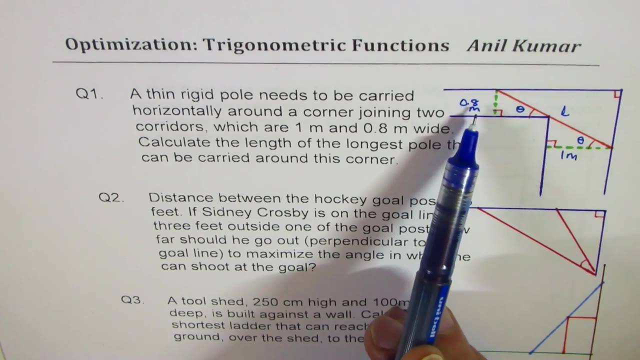 has to be angle theta also. Now you can find the maximum length of the pole using trigonometric functions, correct? Now this length is combination of these two. You can define those as X and Y, write them in terms of the given dimensions and differentiate. 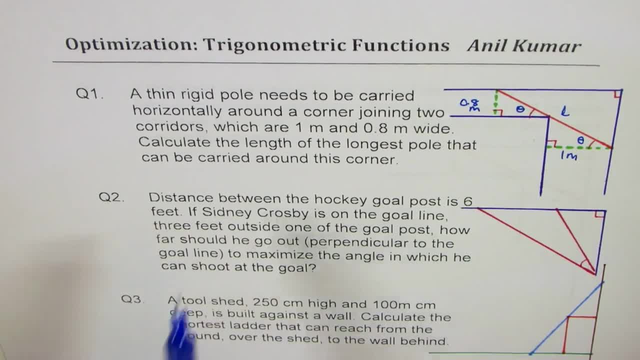 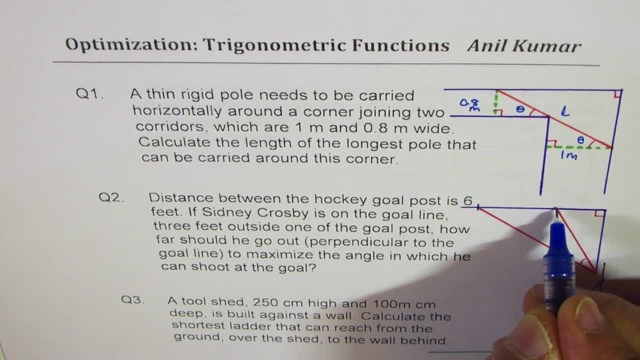 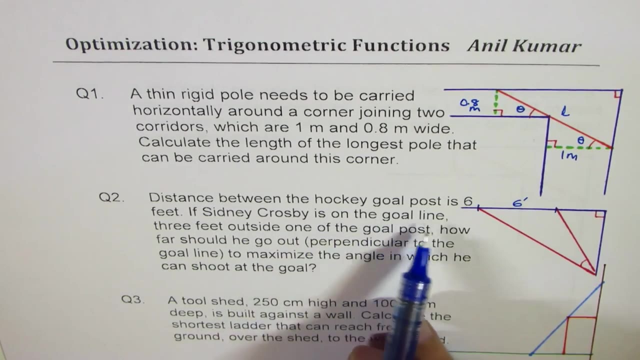 to get the answer correct. Question number two: Distance between the hockey goal post is 6 feet. So let's say this is the hockey goal post, So this distance we are taking 6 feet. If Sidney Crosby is on the goal line 3 feet outside, that is 3 feet. 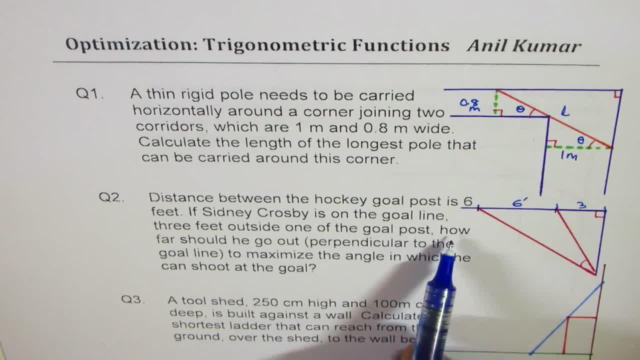 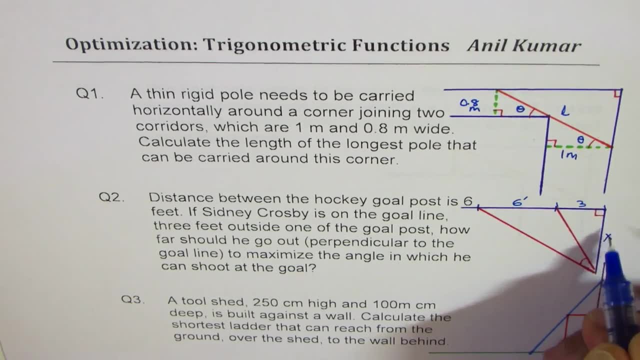 outside the goal line of one of the posts. how far should he go out perpendicular to the goal line? That means this distance. So we are taking this distance as X right To maximize the angle in which he can shoot at the goal. So that's the angle theta, in which 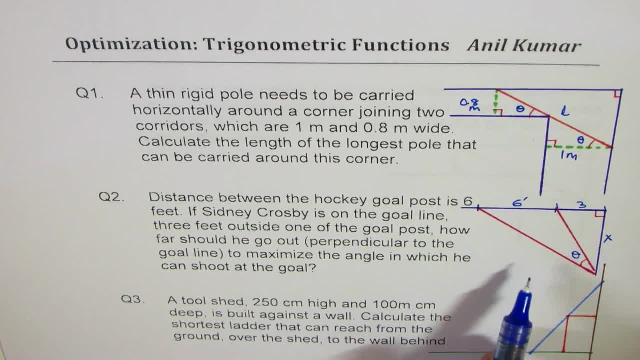 he can shoot at the goal right. When the diagram is before you it's kind of simpler to understand the question and solve it. But in the test you may not get this diagram, So try to think how you can visualize the situation. make. 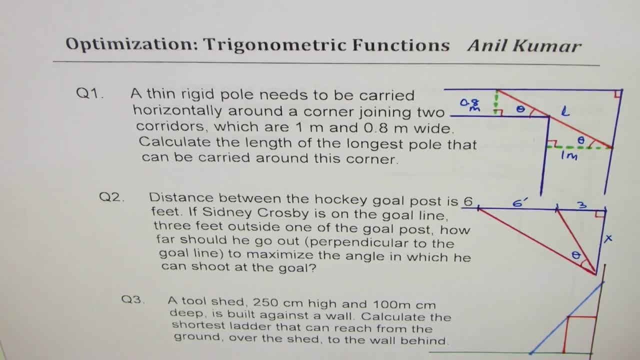 a diagram and then solve it right. Question number three: here is a tool shed 250 centimeter high and 100 centimeters deep is built against a wall. Calculate the shortest ladder that can reach from the ground over the shed. So the length of the ladder is L. This is the shed, which is 250 centimeter high. So 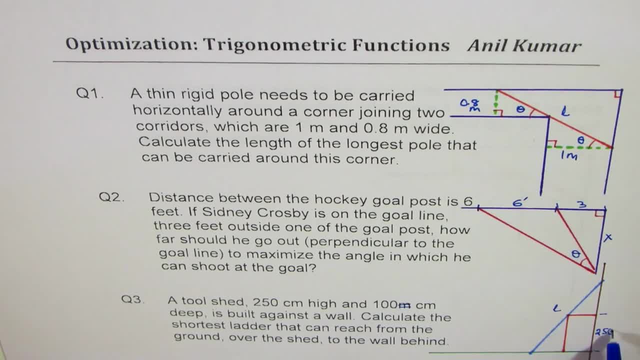 that height is given to us as 250 in centimeters and 100 centimeters deep, So that is 100.. Is that okay? And that's the ladder. So these are three questions for you. Try to solve them. Question number three: here is a tool shed, 250 centimeter high and 100 centimeters deep. 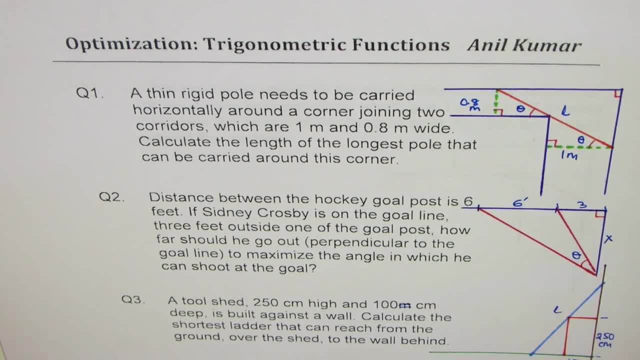 is built against a wall. Calculate the shortest ladder that can reach from the ground over the shed? Question number three: here is a tool shed 250 centimeter high and 100 centimeters deep. So that is one of the questions that we are going to solve today. 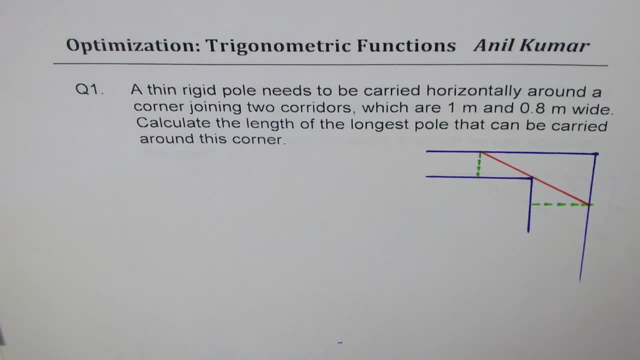 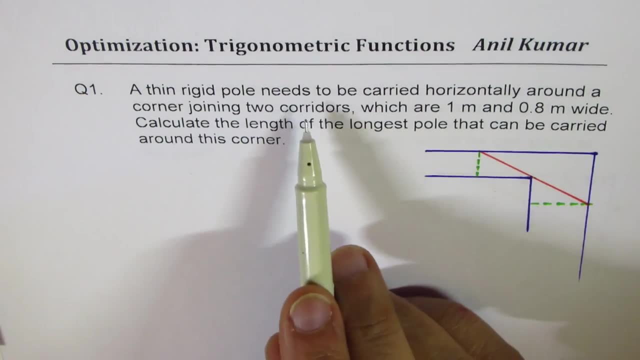 They'll help you to understand most of the concepts. Now let's look into the solution of question number one. A thin, rigid pole needs to be carried horizontally around a corner joining two corridors which are one meter and 0.8 meters wide. 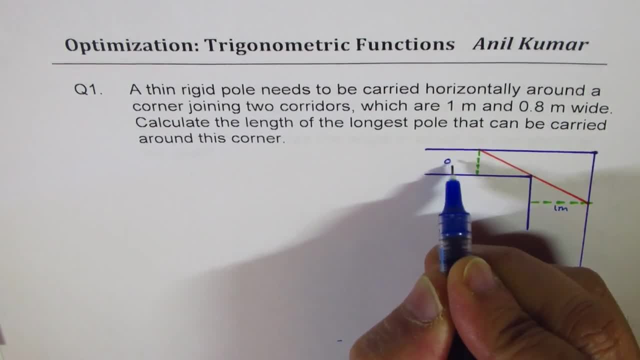 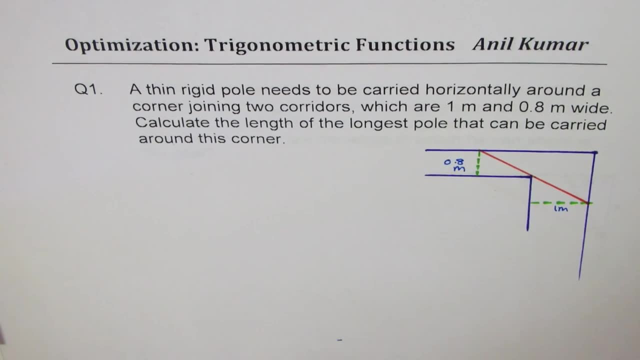 So let's say this is one meter and this is 0.8 meters. Calculate the length of longest pole at half of this with the dye amount, the upper and lowerně of each pole, and separate the columns pole that can be carried around the corner. So that's the corner we are looking into. 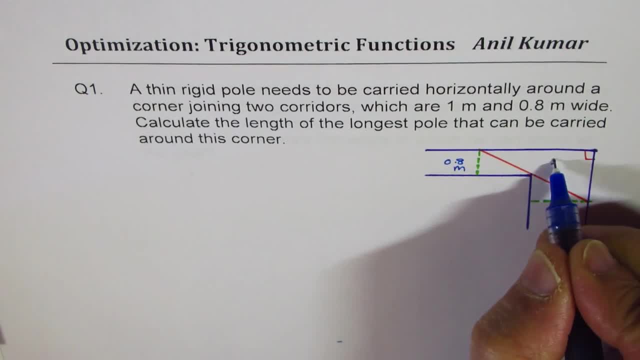 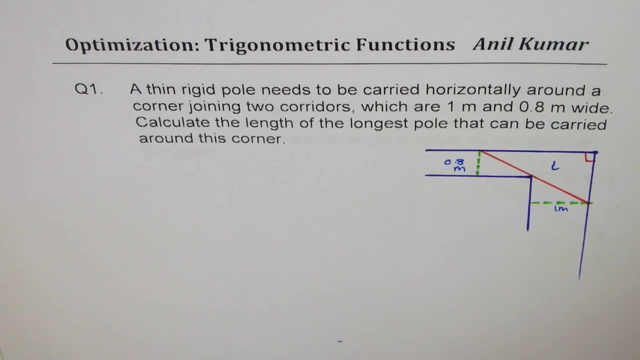 So let's say that the length of this pole is L. Now, in this particular case, what we can do is we can think about the angle made by the pole as theta and we can write L as combination of these two lengths. So let me call these lengths as x and y. Okay, so we 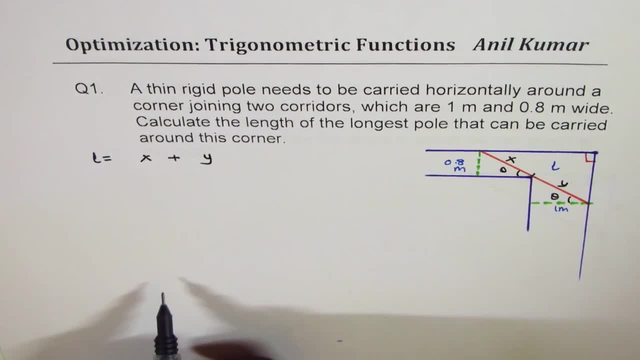 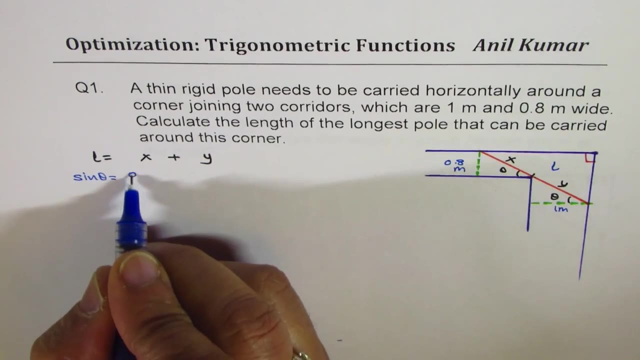 can say: L is combination of x and y. Now what is x equals to? Now, what is theta? So we can say in this triangle: sine theta is equal to zero point eight over x, and that gives you x is equal to Fabian Formas. 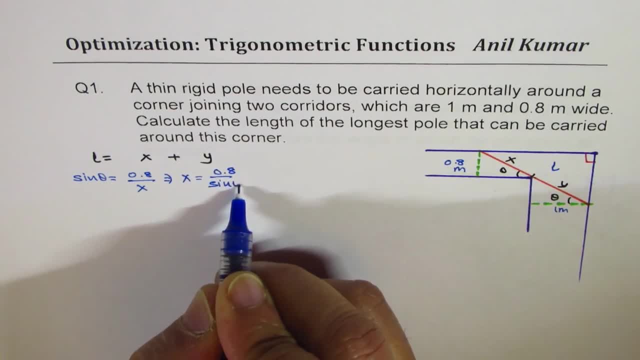 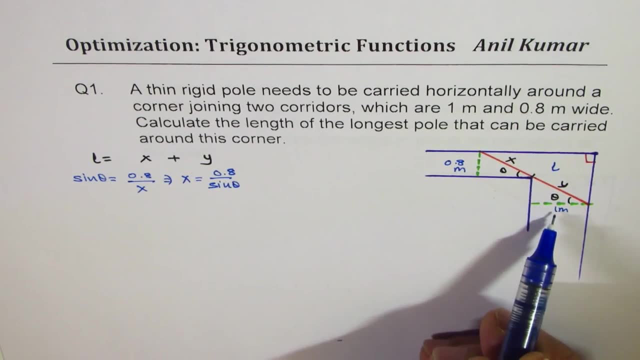 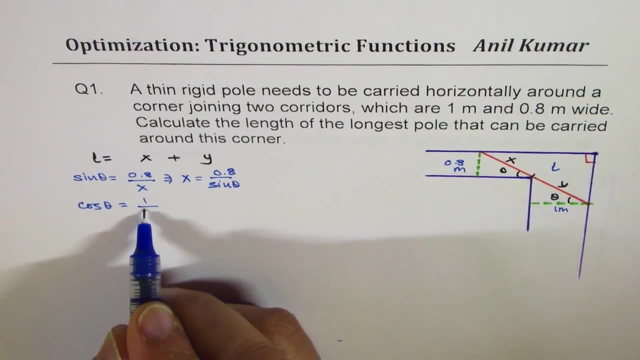 0.8 over sine theta correct. now, similarly, in the smaller triangle, we can write: since we are given the adjacent side is good to write in terms of cosine theta correct, which is 1 meters over y. so that gives you that that y is equal to 1 over cos theta correct. so now we can write what length. 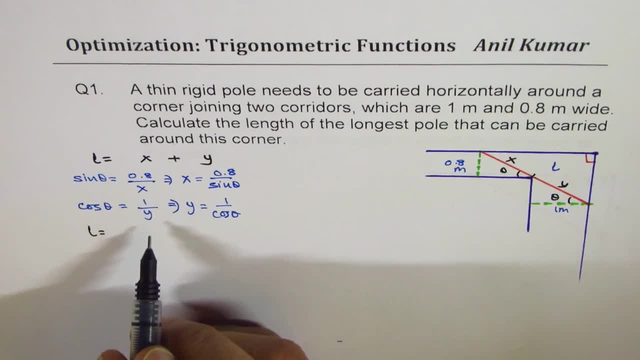 L is in terms of sine and cosine, so L is 0.8 over sine theta plus 1 over cos theta. to maximize, we need to look into the first derivative. so let's find derivative of this function with respect to theta, since as our variable right. so basically we have written length as a function of theta. do you see that? 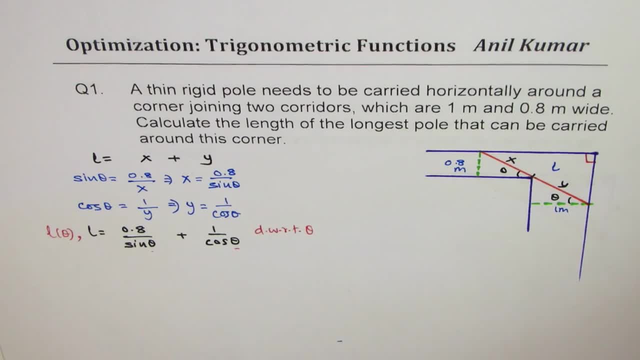 so we can differentiate both sides with theta. so we get d l, d theta equals 2. now here we'll apply the quotient rule. so we get sine square theta in the denominator derivative of sine theta is cos theta, but with a negative sign because this is to the power minus. 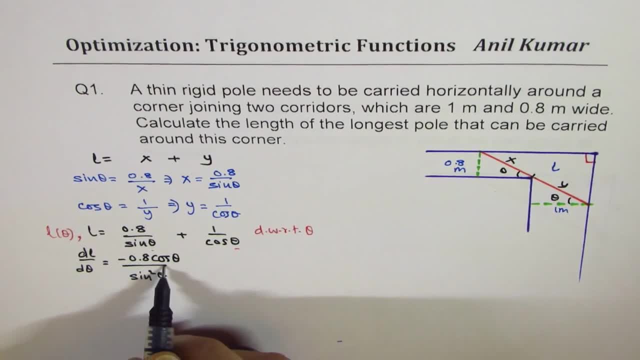 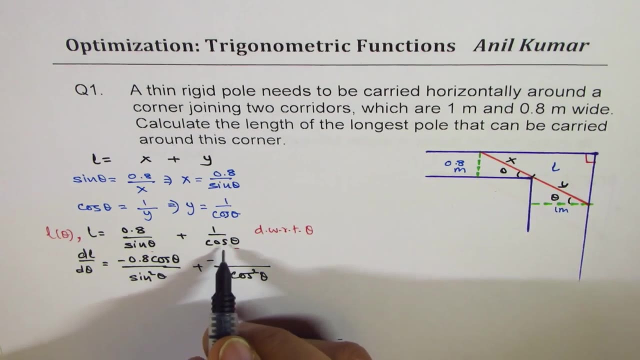 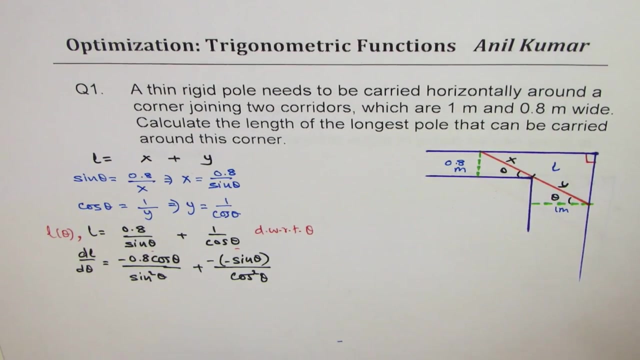 1, 0.8 cos theta. okay, and here we get cos square theta, so minus, because when you take this, it is to the power of minus 1 right, and derivative of cos theta is minus sine theta. so that's what you get. you now for the critical number. so let's find the critical number for the critical number. 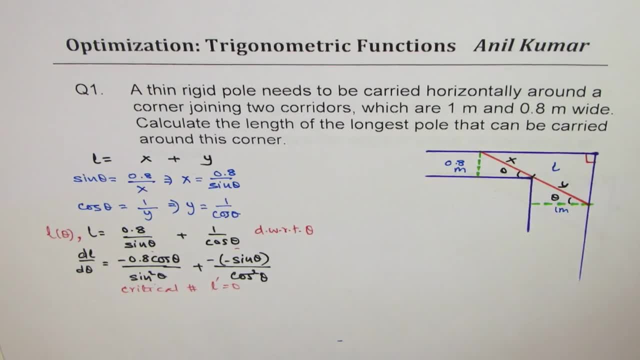 l dash should be equal to 0, the derivative should be 0, that is to say now the whole thing should be equal to 0, so we'll code this as equal to 0. let's take common denominator which is sine square theta times cos square theta. when you cross multiply we get minus 0.8 cos cube theta. 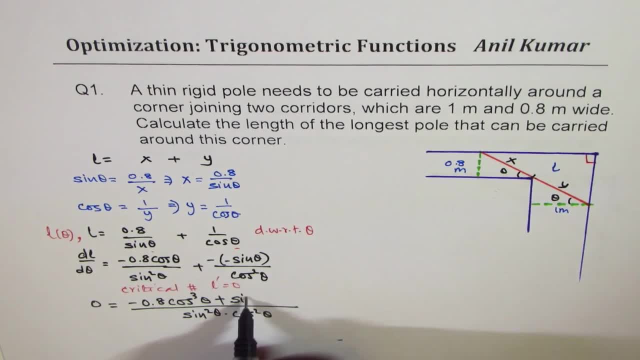 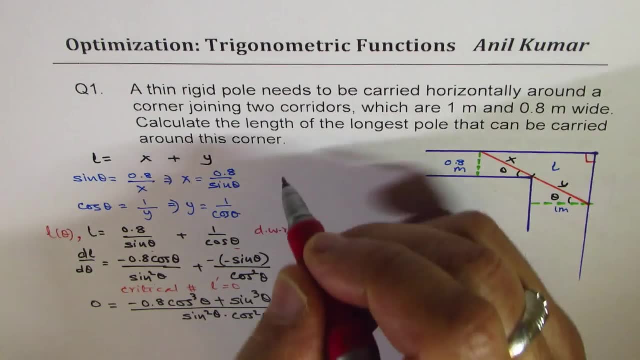 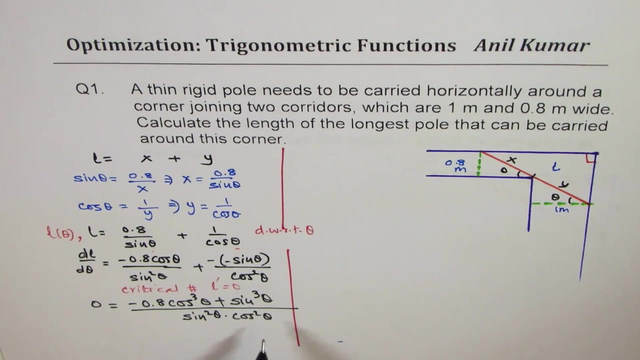 that minus minus becomes plus sine cube theta correct. now to solve further, let me take it to the right side. we have some space here and then work it out. so for the whole expression to be zero, on the right-hand side, the numerator should be zero, right? so what do you get? taking one of these terms, this is negative, that is. 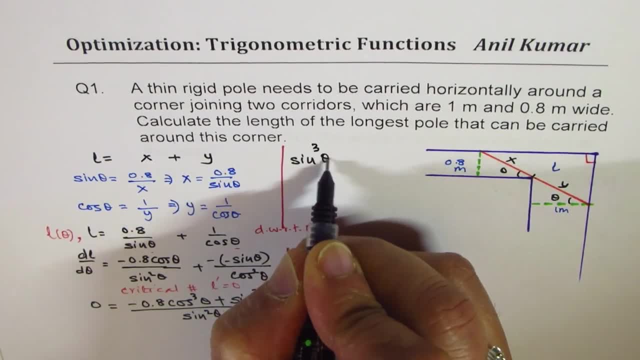 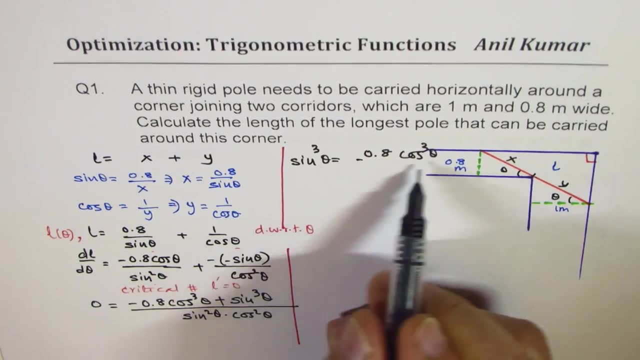 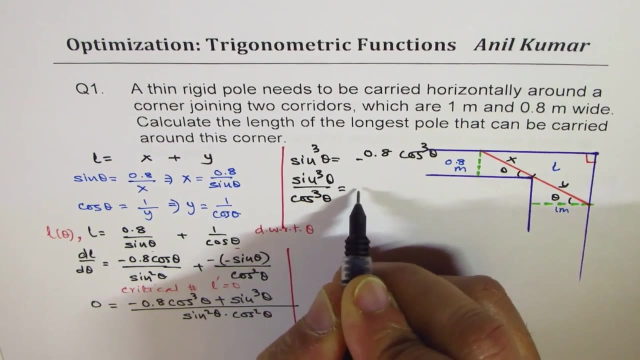 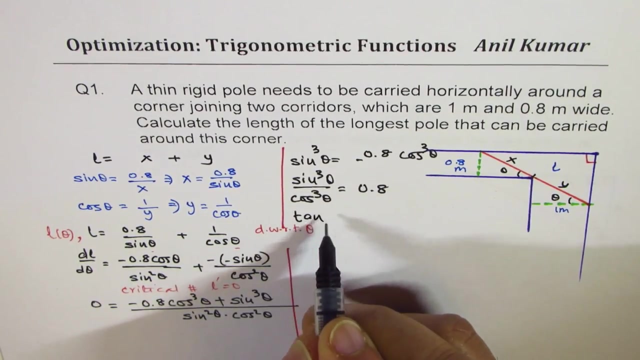 positive. I could write this as: sine cubed theta equals to 0.8. cos cubed theta? now we'll divide both sides by cos cubed theta, so we get sine cubed theta over. cos cubed theta equals to 0.8, and so that is tan cubed theta, right? so tan cubed theta equals to 0.8 and that gives. 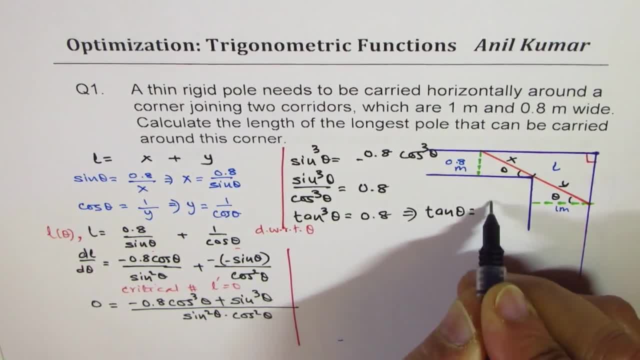 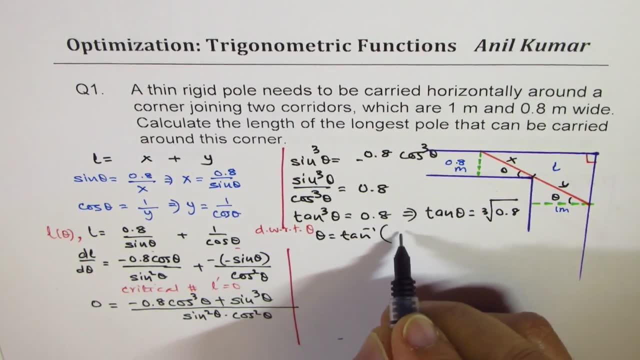 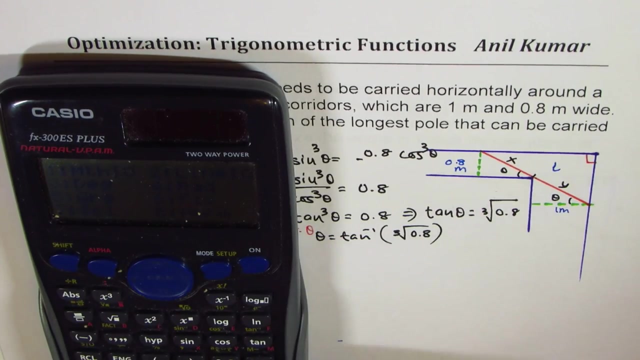 you tan theta equals to cube root of 0.8. so theta equals to tan inverse of cube root of 0.8. so you can use the calculator, set your calculator in radians. well, this particular question you could do in degrees also. but whenever you're working in trigonometry, make sure that your calculator is in. 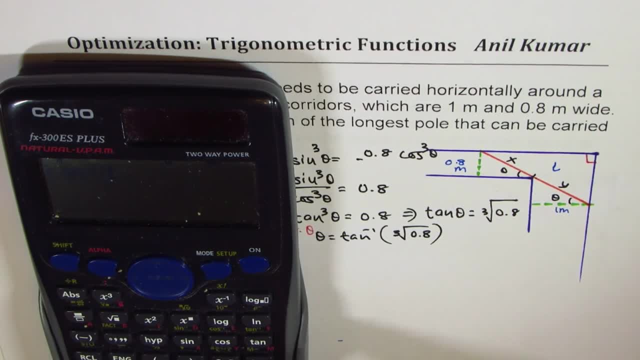 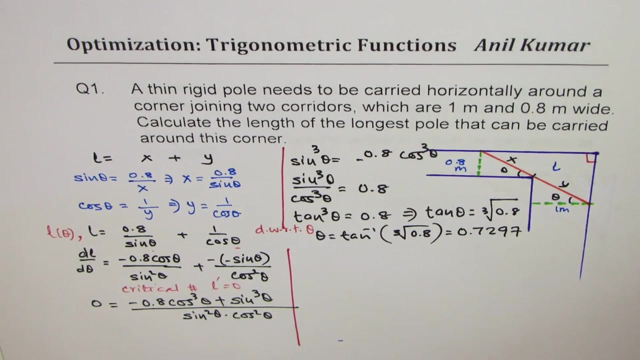 radians. right now, let's find tan inverse of cube root of 0.8. so that gives you the value of theta as 0.7297 right now, this gives you a maximum or not. how do you decide that? well, we could look into two conditions. one is that 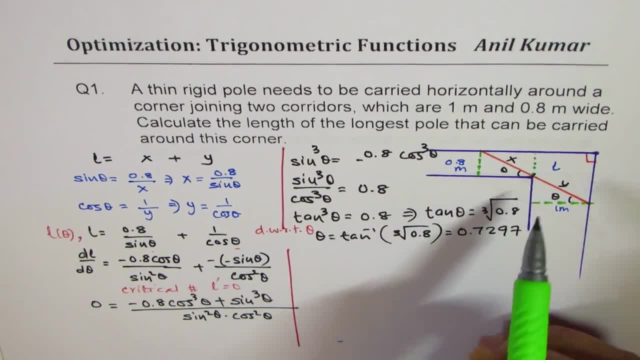 you could take a rod which was like kind of vertical. in that case length is 0.8. you could take a rod which is kind of horizontal. in that case length is 1 meters. so if our answers more than 1 meters, that is maximum. is there, okay? so 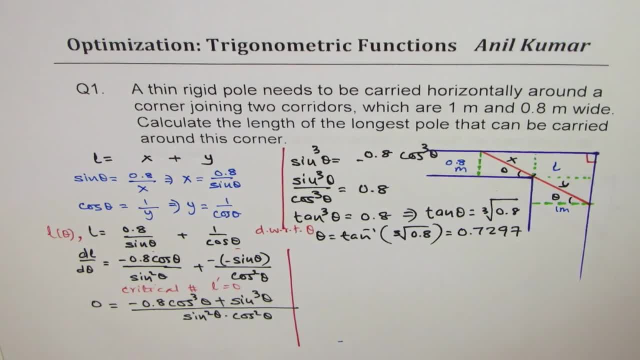 those are the two limits. with that, we will check the value now. right, so what do we get here? is theta to maximize or to minimize, you can say. is this theta n equal to effective Пол이리ך? right, and this is in radians. okay, now let's figure out how much it is. we'll 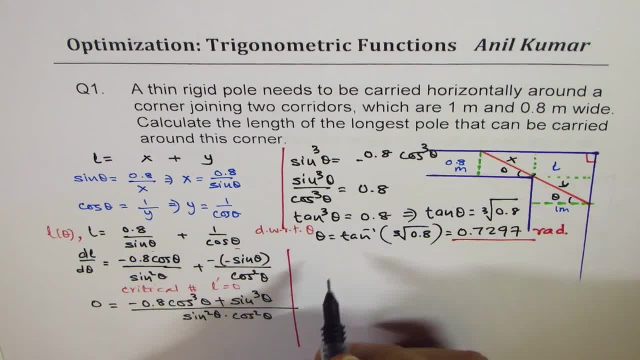 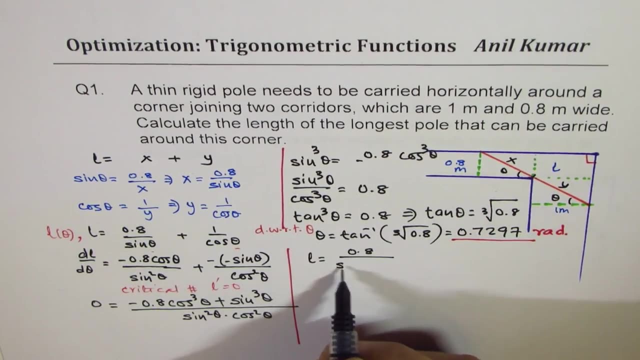 just substitute the value and calculate so. so length is X, is 0.8 over X, which is, I mean, 0.8 over sine of theta, which is sine of this value. 0.7297 plus 1 over cos of 0.7297 is ok, so we'll just calculate this value, so we have 0.8. 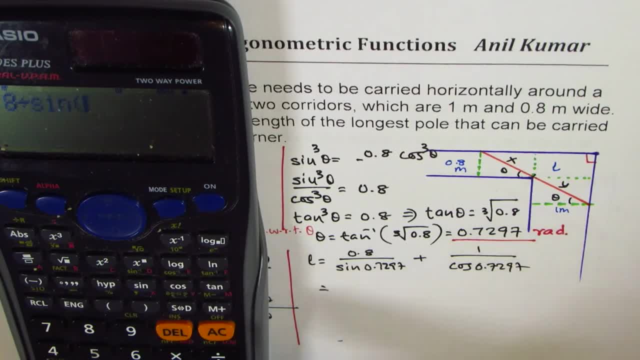 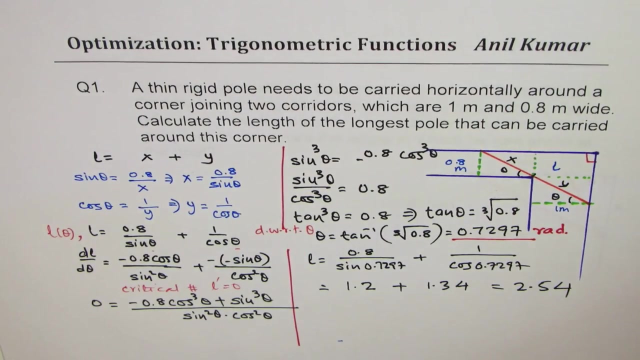 divided by sine of 0.8, 0.7297, which is equal to 1.2, plus we have 1 divided by cos of 0.7297, which is equal to 1.34. so when you add them up, you get 2.54 as your answer, right, so so? 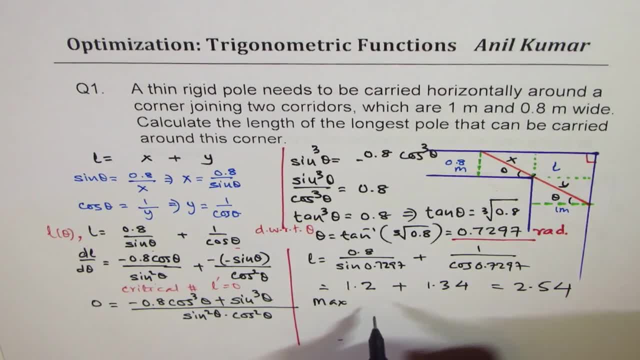 the maximum length: 0.7297, which is equal to 1.34. so when you add them up, you get 2.54 as your answer, right? so so the maximum length, rod length- in this case, is 2.54 meters. is it correct, since it is more than 1? 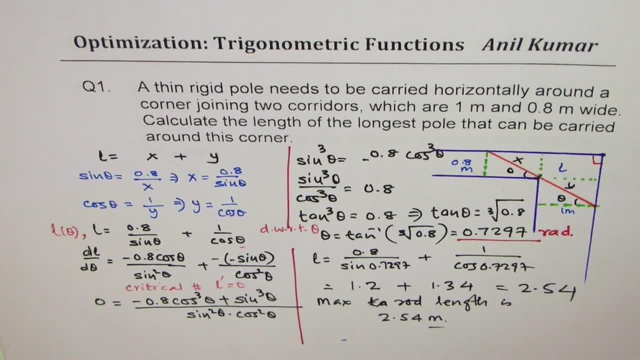 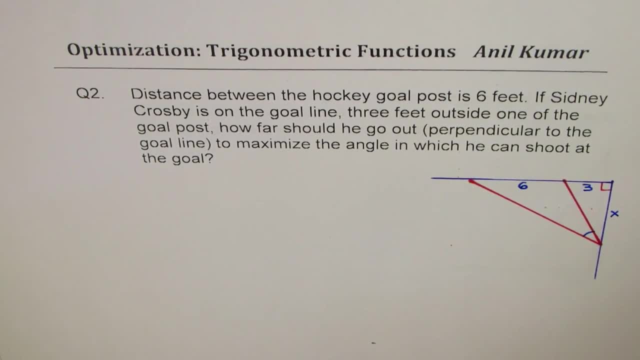 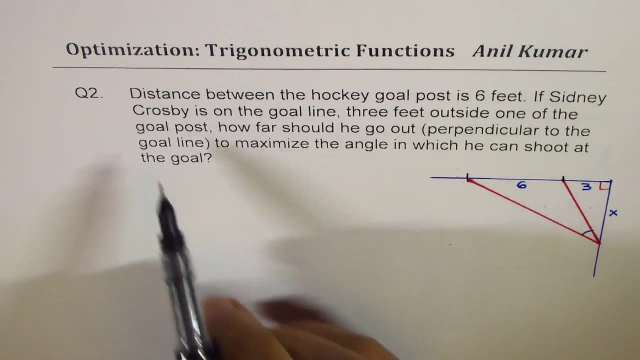 meters, we'll say this is maximum length. right, so now let's move on to the next question, question number two. distance between the hockey goal post is 6 feet. so that's the distance between the hockey goal post. if Sidney Crosby is on the goal line three feet outside one of the goal post, how far should he go out? 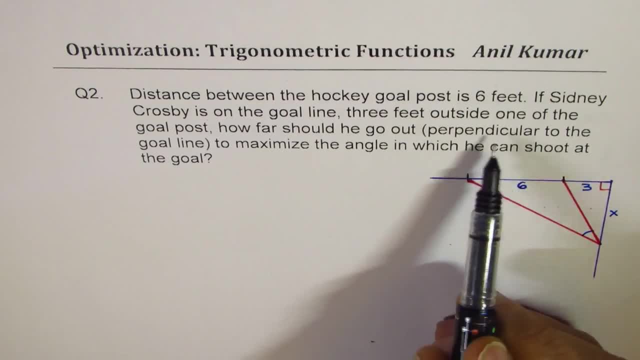 that means in this direction, perpendicular to goal line, to maximize the angle in which he can shoot at the goal. so that's the angle, theta, which we want to maximize. now, this is really a very interesting question and you have to use knowledge of exterior angles to solve this kind of question. so let's try. 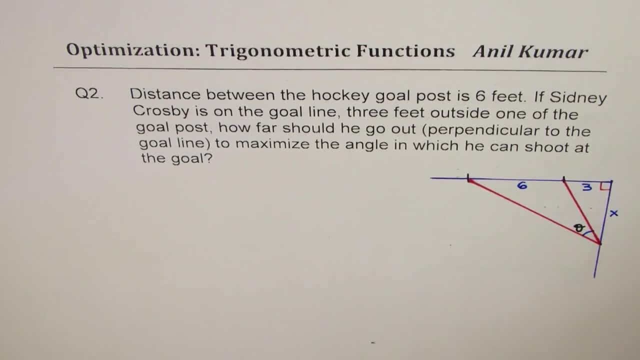 to understand. so let us say that we have. we have to relate this theta. you can actually use cosine law also. but what we will do is will we'll say: let these two angles be alpha and beta. let me call this alpha. we can write this as beta, we can write this as sigma. we can write this as: 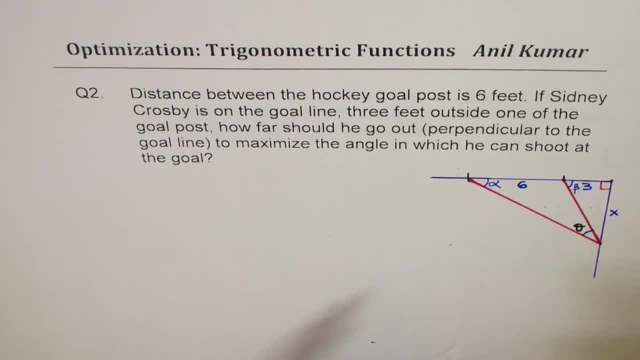 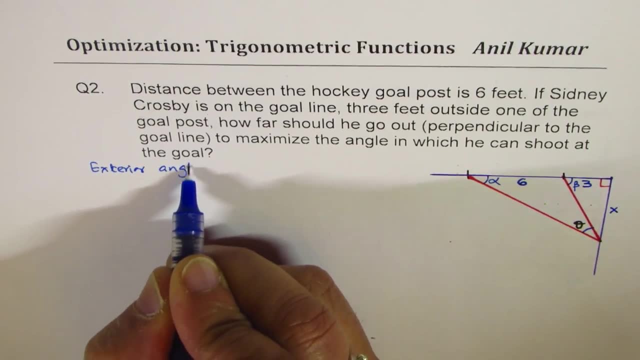 omega. we can write this as delta, we can write this as sigma, we can write this as as alpha, this as beta, that is theta right. So the exterior angle beta is equal to some of these two angles: alpha plus theta right. So that gives you: 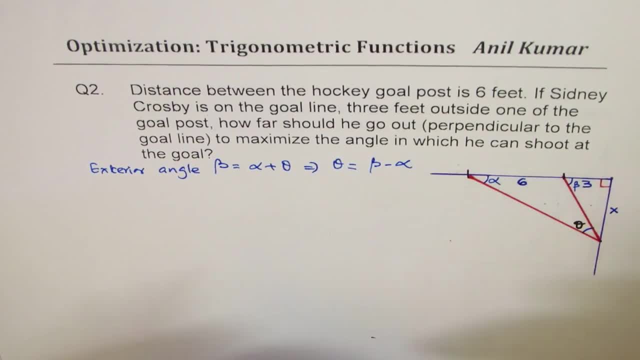 that theta is equal to beta minus alpha. Does it make sense to you, Right? So we'll follow the angles rather than finding a side. You could actually find the sides, apply cosine law also and solve this question, Is it okay? You can do that. 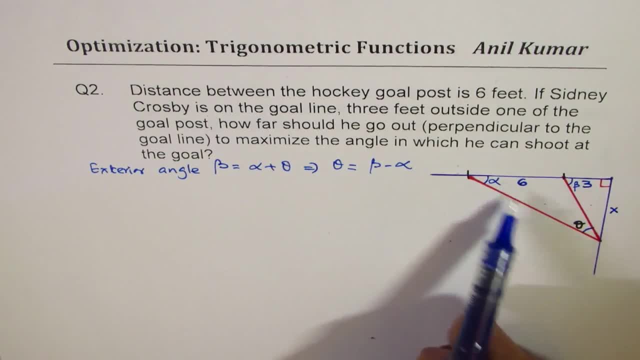 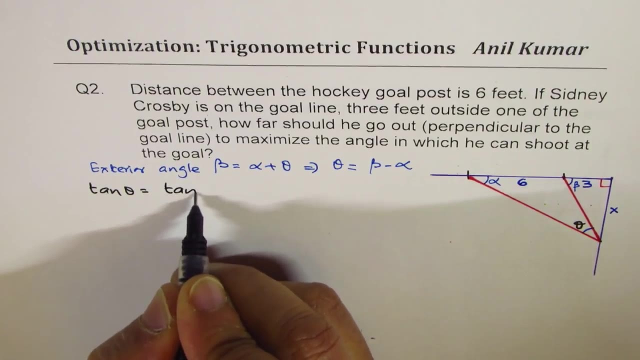 Now what we did was we just related this angle with all this theta. Now what is tan theta equals to? So let me write down: Tan theta could be written as: tan of theta is beta minus alpha, beta minus alpha. Do you see that? 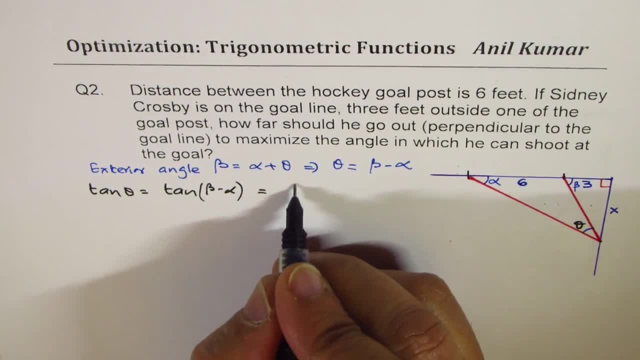 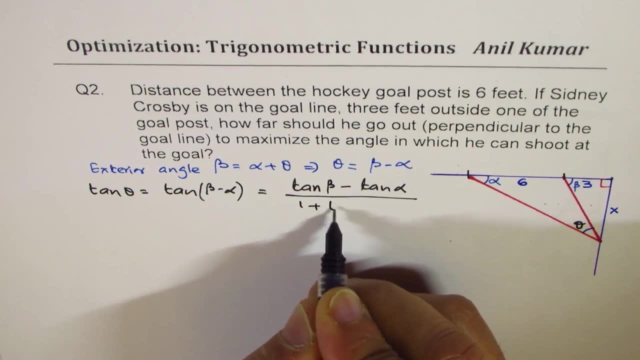 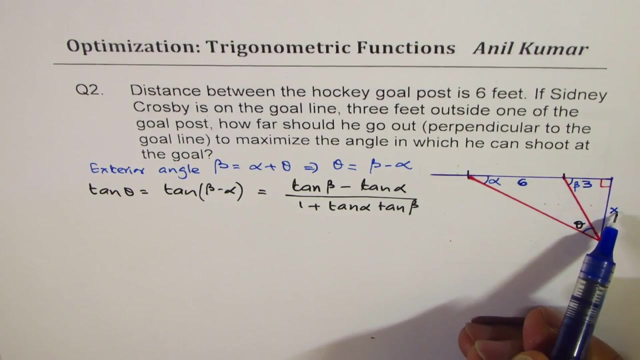 And you know the combination Compound angle formula. you could expand this as tan beta minus tan alpha over 1, plus tan alpha, tan beta. Perfect, right Now, what is tan alpha and what is tan beta? Let's look into this diagram once again. Alpha means opposite side over base. 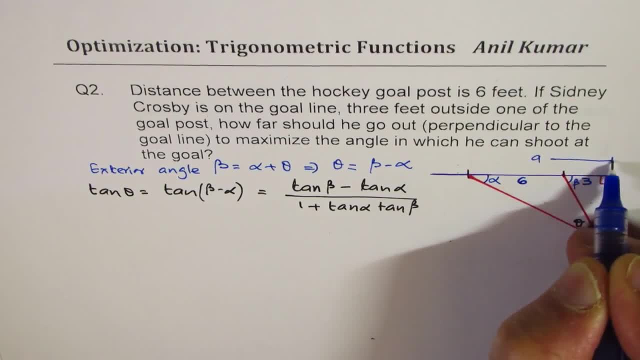 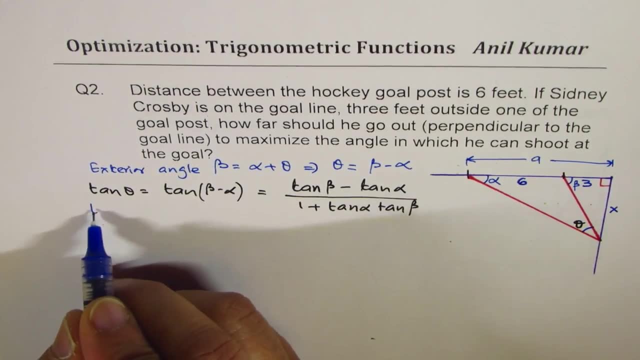 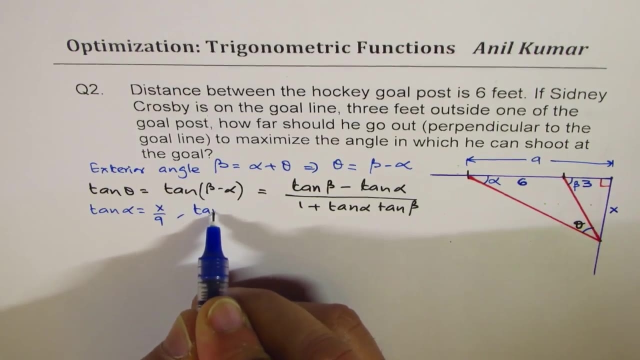 which is 6 plus 3.. So the total length here is 9,, correct? So tan alpha is- we can write here first- tan alpha is x over 9, and tan beta is the smaller triangle: x over 3,, right. 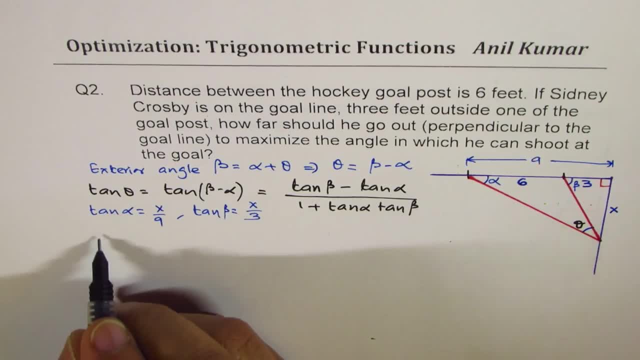 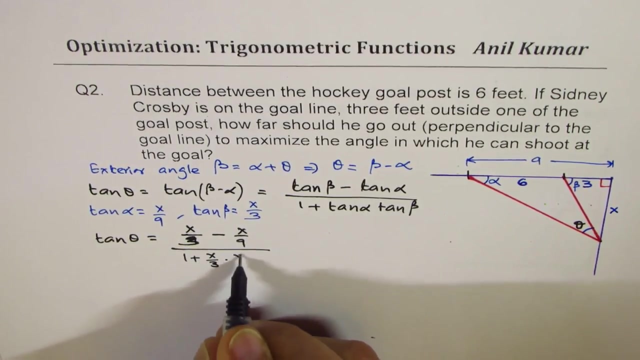 So replace these values here, and so we get tan. theta equals to x over 9, minus- I'm sorry this is beta is x over 3.. So this is 3, and this is x over 9, over 1 plus x over 3 times x over 9,, correct. 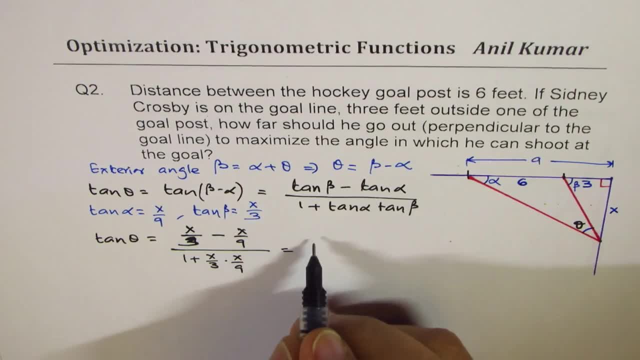 Now, taking common denominators as 9, I could write this as 3x minus x divided by. we took 9 as a common denominator. Here, common denominator is 27,, so we get 27 plus x squared over 27,. right Now this could be written as: tan theta equals to 9 and 27.. 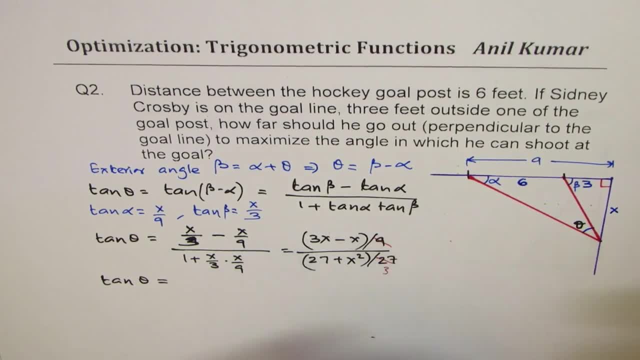 You could cancel three times. So divide means it comes on the top. So we get three times within bracket. 3x minus x is 2x and in the denominator we have 27 minus plus x squared. So I hope it's absolutely clear. 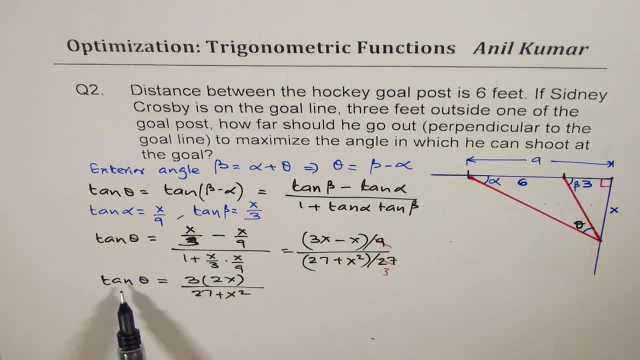 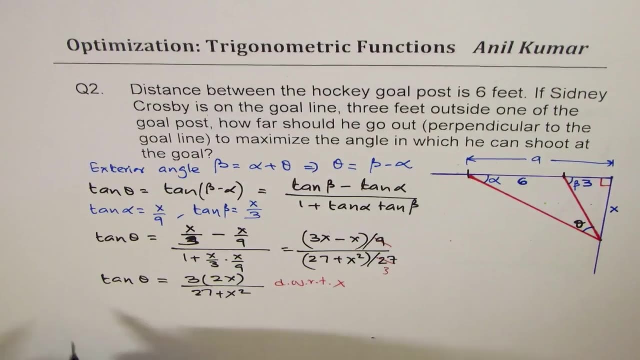 up to now. So what we've done here is we have written in terms of x this expression. We'll now differentiate both sides with respect to x. So what do we get? Derivative of tan theta is secant squared. theta times d, theta, dx, and here we are going to apply the quotient rule. 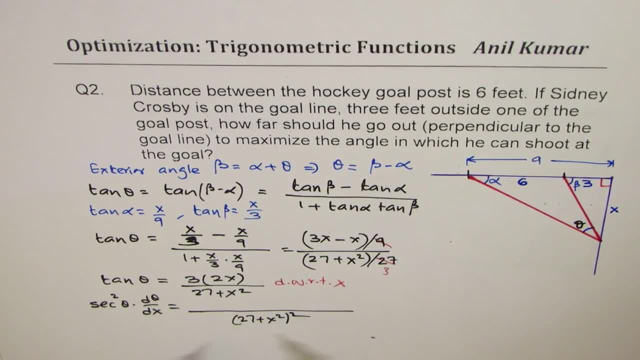 So we get 27 plus x squared, This is 6x. Derivative of 6x is 6.. 6 times 27 plus x squared, minus 6x times derivative of denominator, which is 2x, And for a critical value, this should be equal to 0, right. 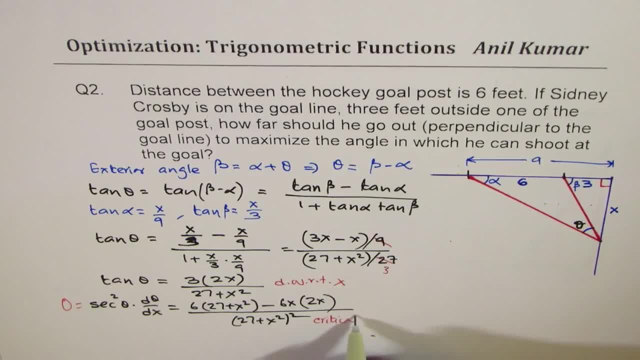 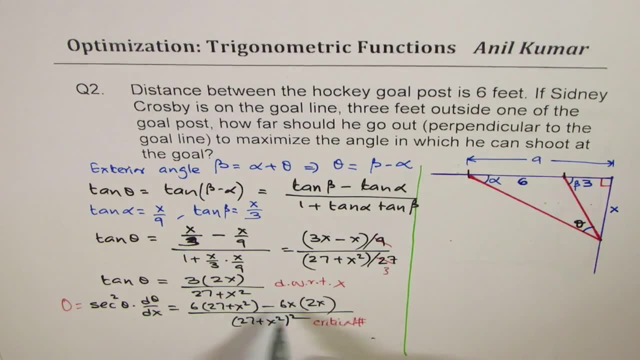 For a critical number, First derivative should be 0, right, So now we'll find x, value for which the critical number is achieved. That means the numerator is 0.. Is that okay? So now we'll just solve the numerator. 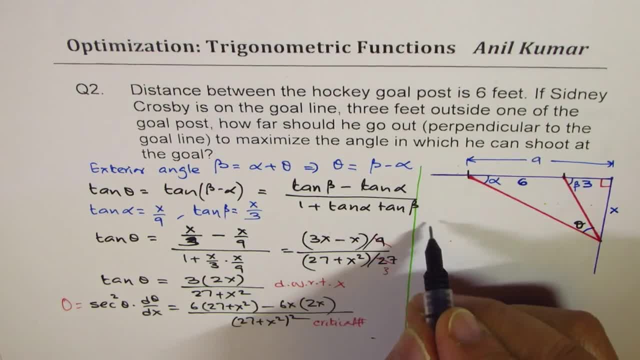 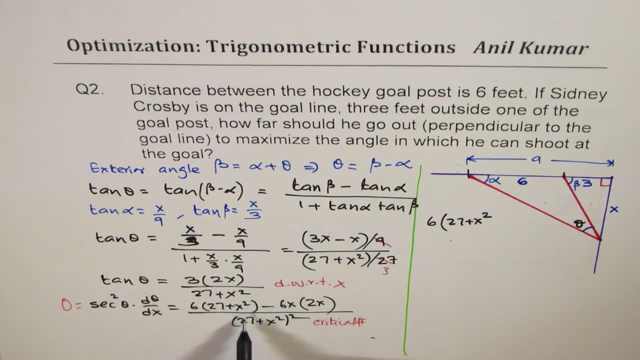 We can take 6 common. That should be 0, right? So we have 6 common. We have 27 plus x squared and here 6 common. So we get 2x minus 2x squared. 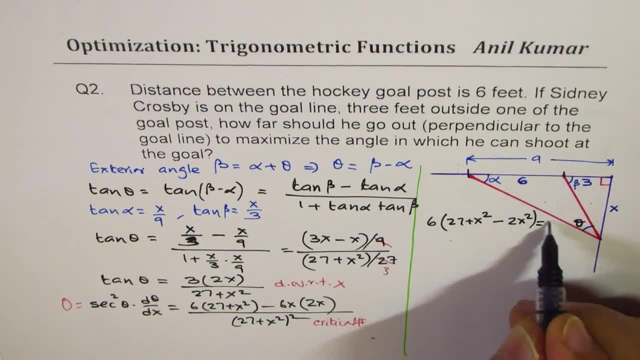 We took 6 squared, So we get 2x minus 2x squared. This is 6 common. okay, That should be equal to 0.. So that means 27 minus x squared is equal to 0, or x is equal to square root of 27,. right, So that is the value of x. 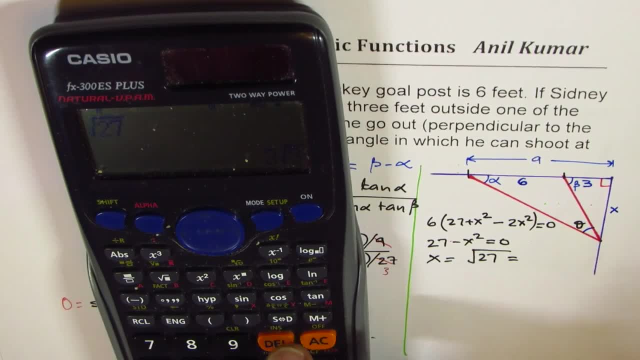 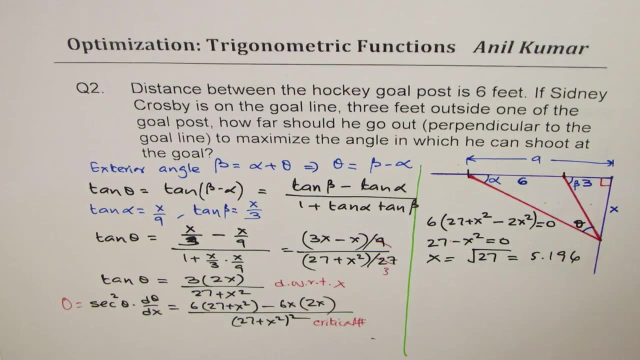 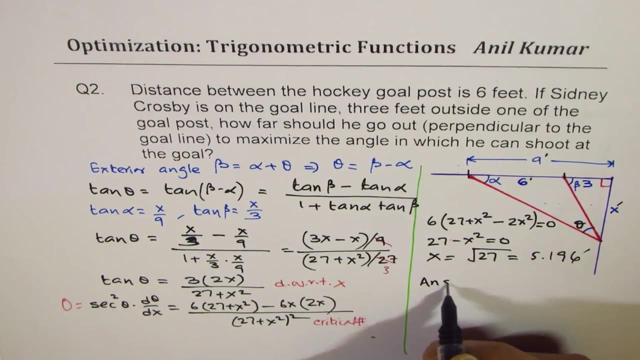 Square root of 27 is equal to 3. square root 3 in decimals is 5.196.. 5.196.. So all are in feet, right, All are in feet. in this case, To maximize, the angle x is equal to, you can say, approximately 5.2 meters. Perfect. 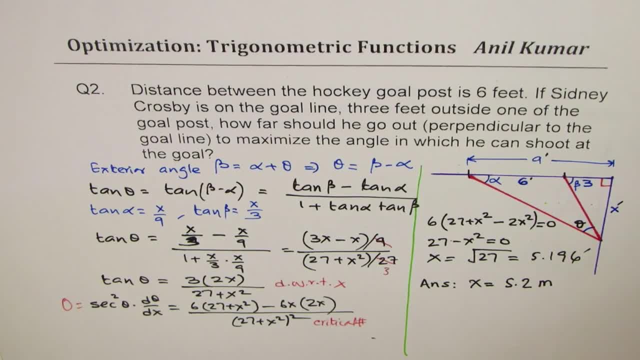 So that is how you can actually solve this question. Now, whether this is a maximum or not, how do we figure this out? Well, we can decide It reduced to how much. 6 was common, right 6, and within bracket we had 27 minus x squared. 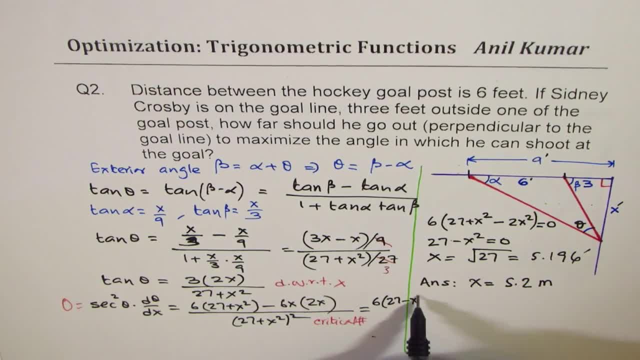 So let me write down 6 times 27 minus x squared, and the denominator is 27 plus x squared, whole squared, correct? So we can take a critical. This is our critical number, right? So this is a critical number, which is 5.2 meters. 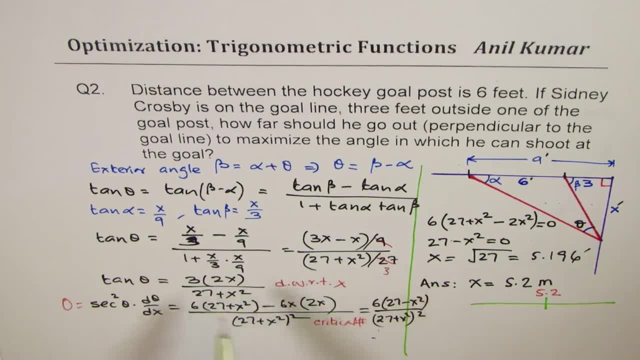 So we let us find the. if I take a value which is, let us say, on the right side, if I take a value which is 6, and on the left side we take a value on 4,, correct? So if I substitute? 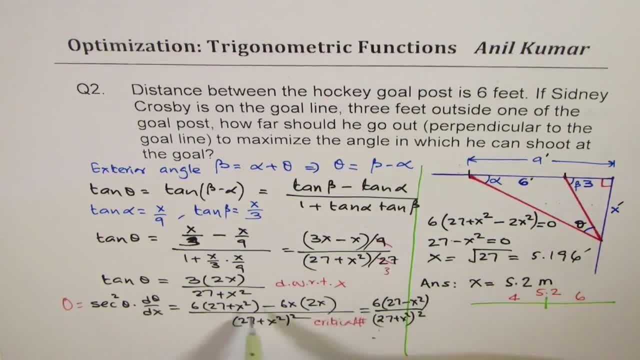 in this value. basically, only this value is to be checked. So if I substitute a value, 4, I get positive. Do you see? This is positive. So we are analyzing secant square theta, but secant square theta is always positive, perfect, This is always positive and we are. 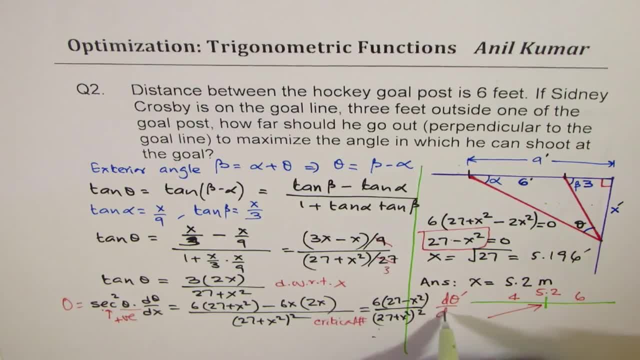 analyzing d theta dx. Let me write d theta dx. So if I substitute 4 here for x, I get positive value. and if I substitute 6, then x squared is 36, you will get a negative value right. So, analyzing the first derivative, we can ensure that this value will give us. 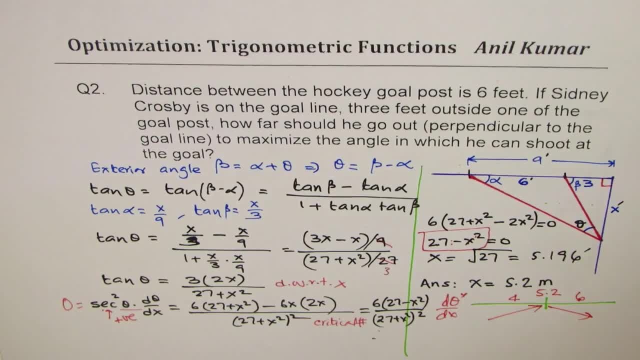 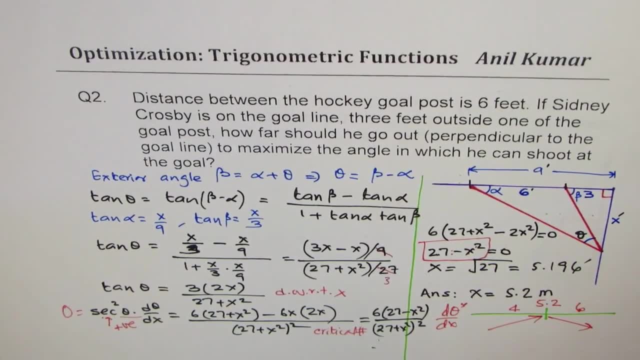 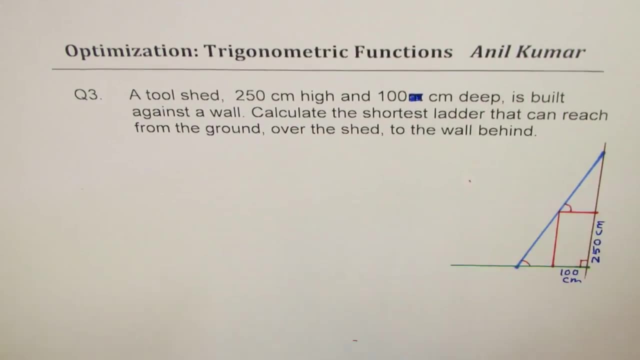 a maximum angle. That is the important part, right? Okay? So I hope that is absolutely clear. Now let us move on to solution of question number 3.. Question number 3. A tool shed 250 centimeter high and 100 centimeter deep. so that is the. 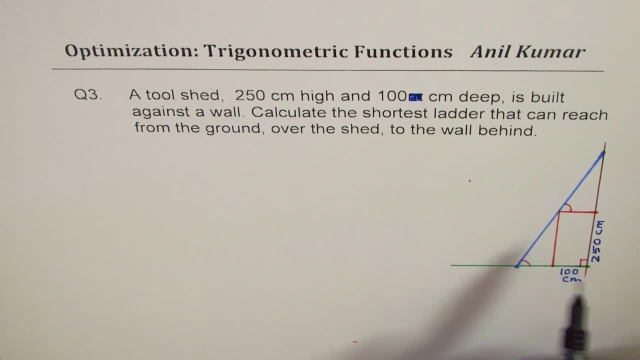 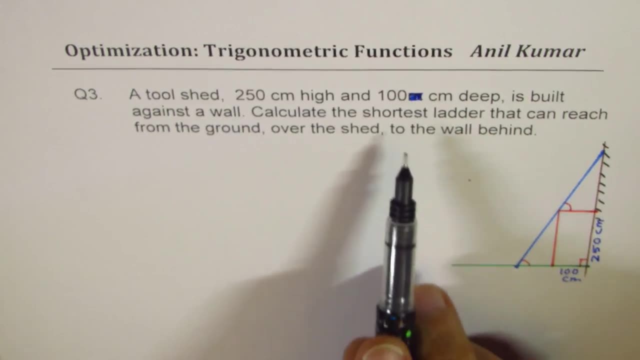 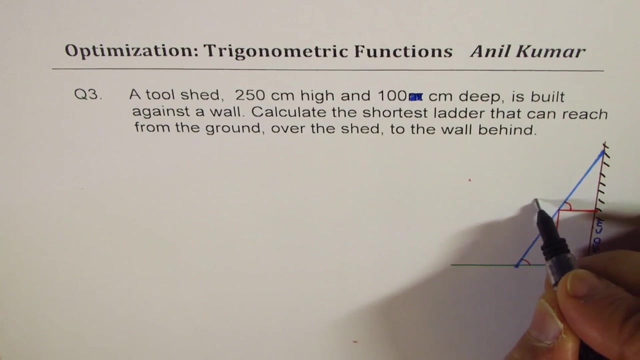 tool shed, 250 centimeter high, 100 centimeter deep, is built against a wall, So that is the wall. Calculate the shortest ladder that can reach from the ground over the shed to the wall behind. So let this be the shortest ladder. So, as we have done in most. 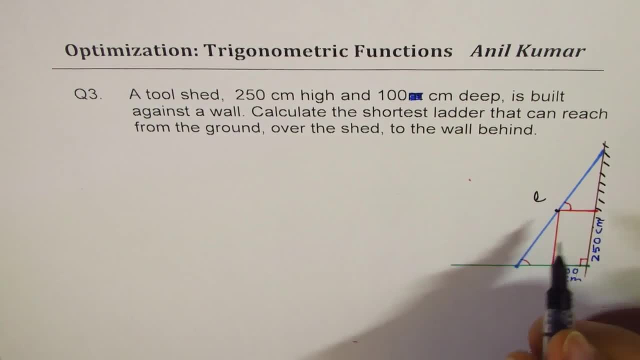 of our questions in similar kind. we will split this length into two values, which is x and y, and we will keep this as theta perfect. So I hope now it is very clear how to solve it. I would like you to actually pause the video, answer this particular question and 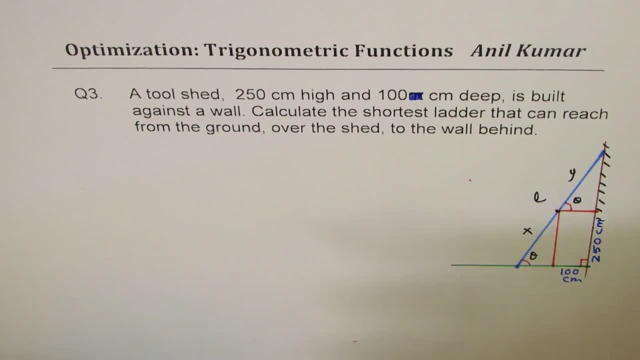 then look into my suggestions. right? So here we can write: l equals to x plus y, but what is x and what is y in terms of theta? Now in this diagram you will notice that this length here is 100, and that height is 250,, right? So this height? 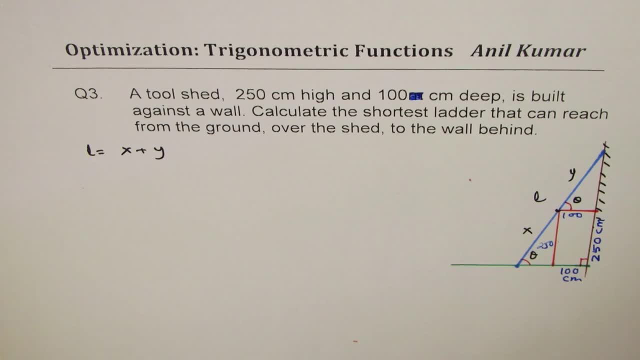 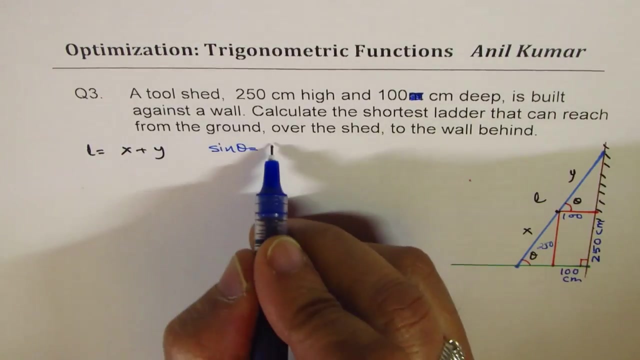 is 250, correct? That should help you to figure it out. So from here it is very clear that if I consider this triangle at the base, then relating opposite side to hypotenuse after y is because if theta is not东so, then x plus y is 150 over h plus beta. That was. 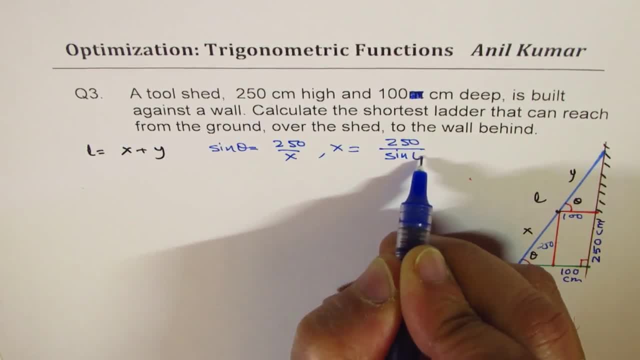 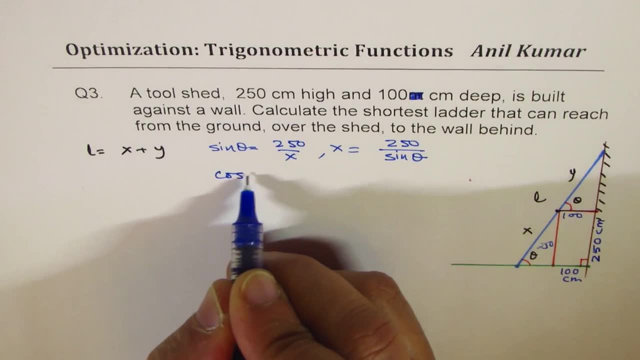 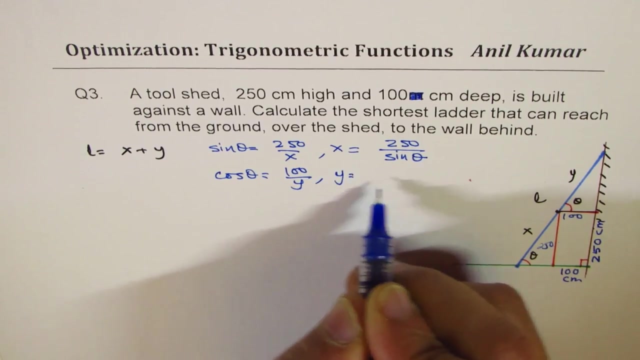 nal Iati and himso And I told you to following flow does not mean cos theta or cos theta over عند either of them. I forgot 100 over cos theta, correct? OK, so we could write length L as equal to combination. 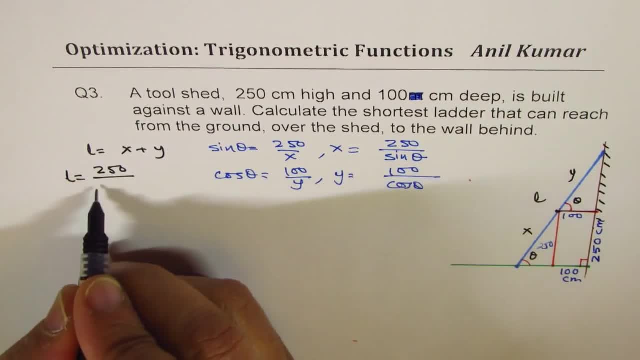 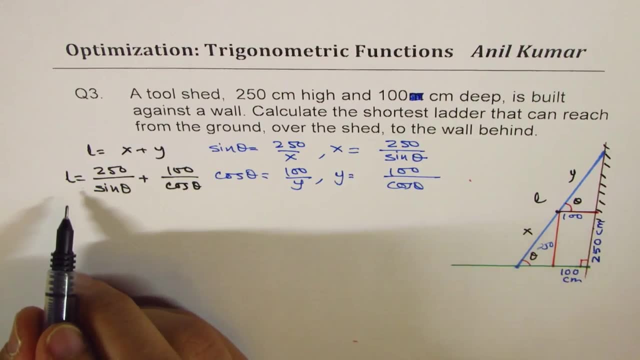 of these two, 250 over sine theta plus 100 over cosine theta And the derivative with respect to theta will give us dL d theta equals 2.. What is the derivative of this? Now I'll use the standard technique which some of my students use. 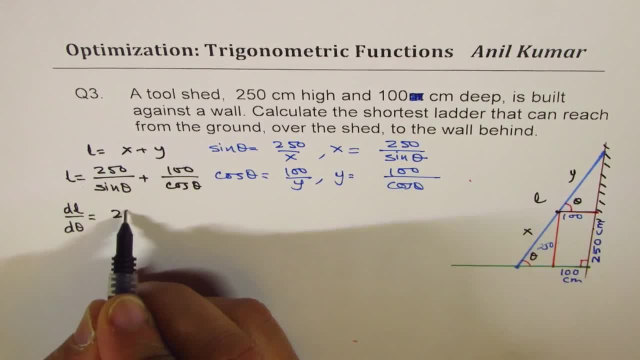 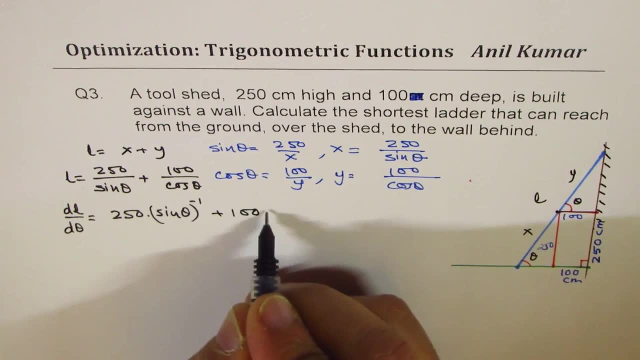 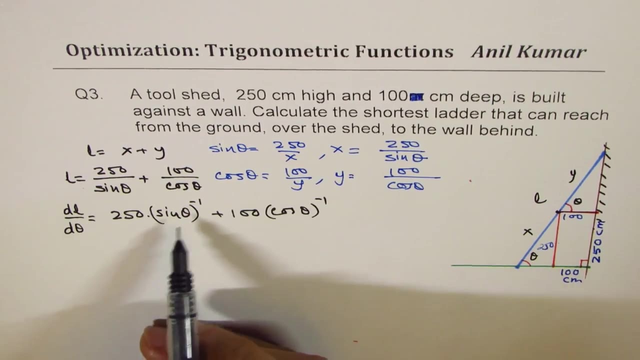 They write sine theta as sine theta to the power minus 1.. So I'm going to use that exercise now. It helps right to do questions in different ways so that all are familiar with what you're solving. So now the derivative could be written: 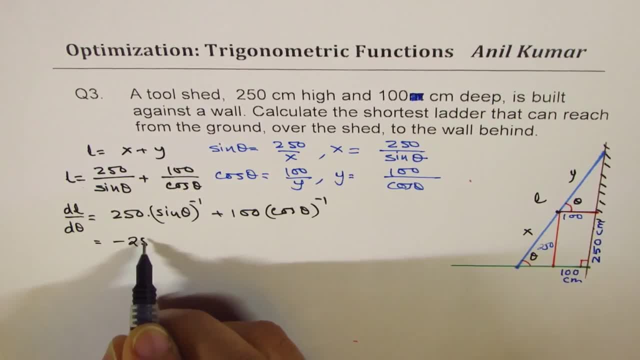 as applying the power rule, We get negative of 250 times sine theta right to the power of minus 2 times derivative of sine theta, which is cosine theta. perfect. Here we get negative 100 times cos theta to the power of minus 2. 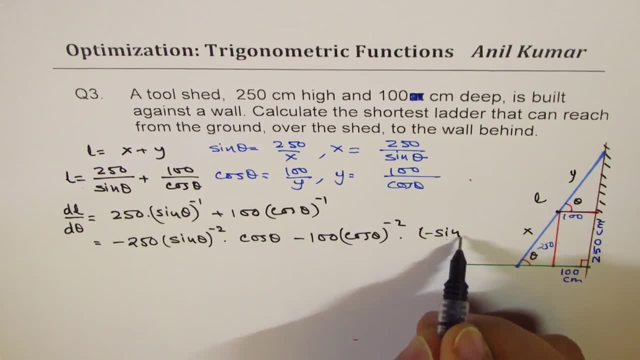 times derivative of cosine theta, which is minus sine theta, perfect. So that gives you. so that minus means it brings it down. So we get minus 250 over sine squared theta times cosine theta. OK, Perfect, OK. So we get minus 250 times sine squared theta to the power of minus 2 times. 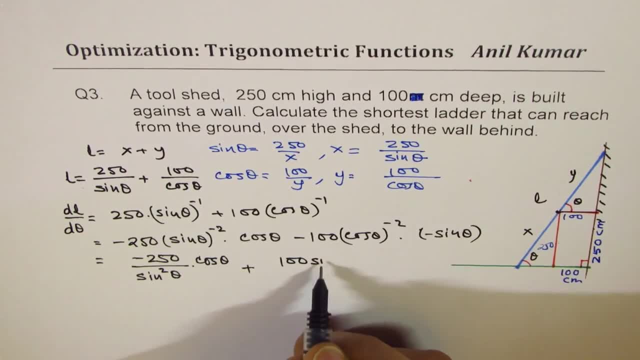 cosine squared theta and here minus and minus makes it positive And we have 100 sine theta in the numerator over cos squared theta. So I hope that step, this step, makes it clear how we did earlier. right, We directly wrote this using quotient rule. 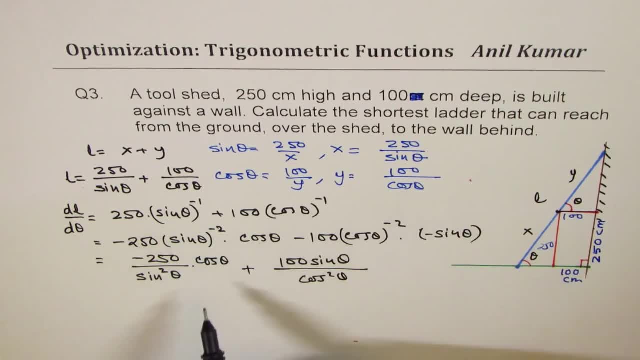 So this time, instead of quotient rule, we rewrite this and use the power rule. OK, So the rest is all same. So dL d theta is this, And we want to equate it to 0 for critical number, right? 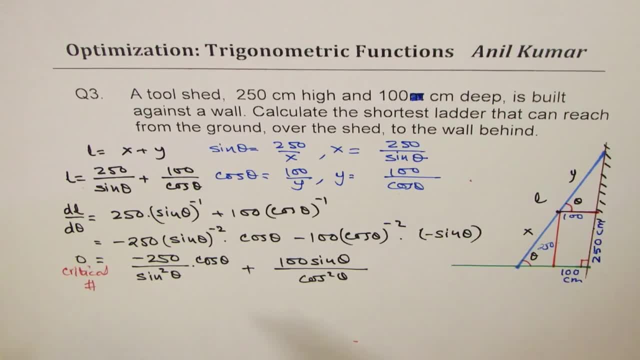 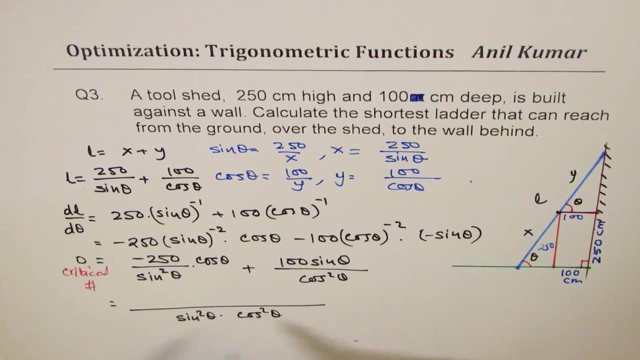 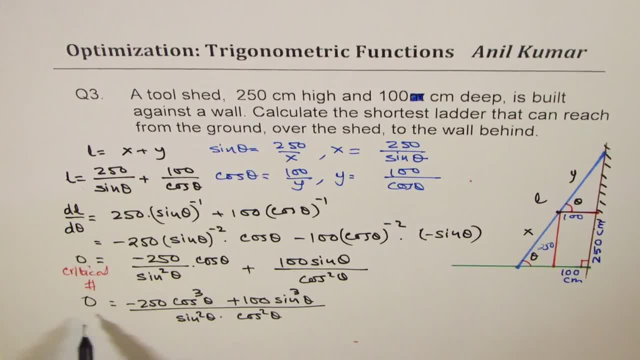 Sine cubed theta, Sine cubed theta, Sine cubed theta, theta. so since that is to be 0, the numerator should be 0, perfect. so let's do that. so we'll make the numerator as 0. that means 100 sine theta. sine cube theta should be equal. to bring it to the. 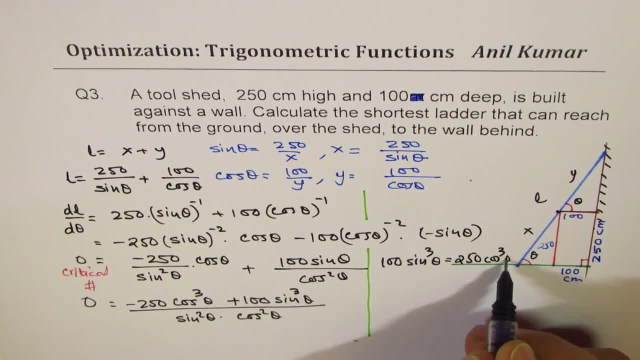 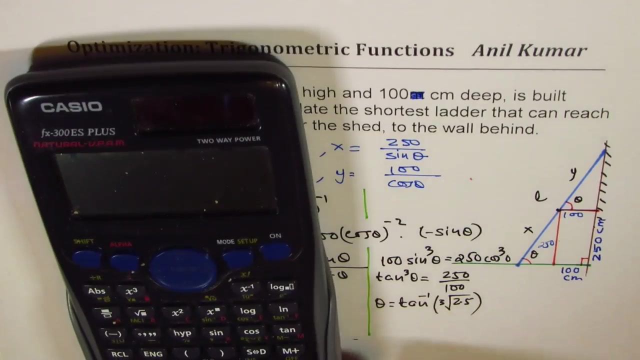 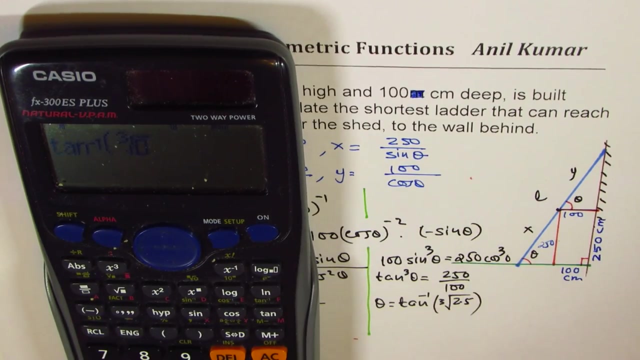 other side 250 cos cube theta. dividing we get tan cube theta equals to 250 over 100. so theta equals to tan inverse of cube root of 2.5. is it so? that is the value of theta? this time theta is tan inverse of cube root of 2.5, which is equal to zero point nine three five. 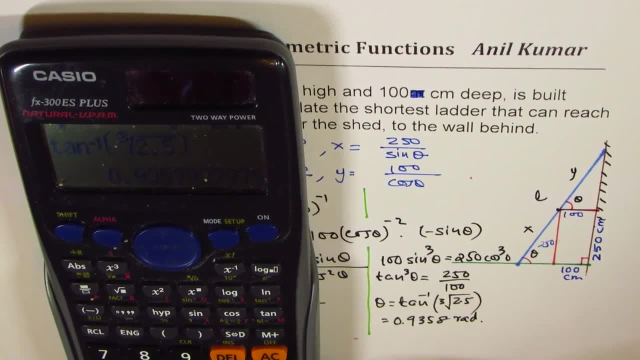 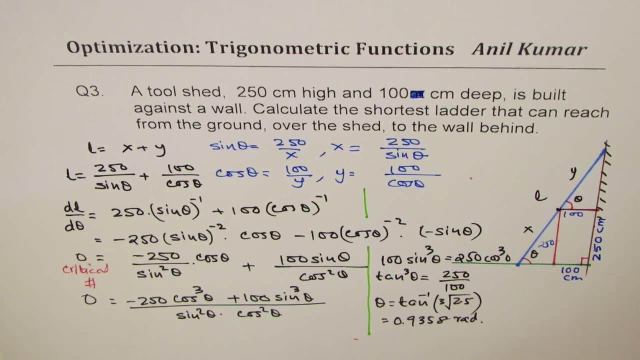 let me write it right: radians. so ensure that your calculator is in radians. you can use degrees, but that will be discouraged in calculus. as you know, the limit of sine theta over theta is valid only in radians, not in degrees. so always work in radians, perfect, okay, now we know this is shortest. why? 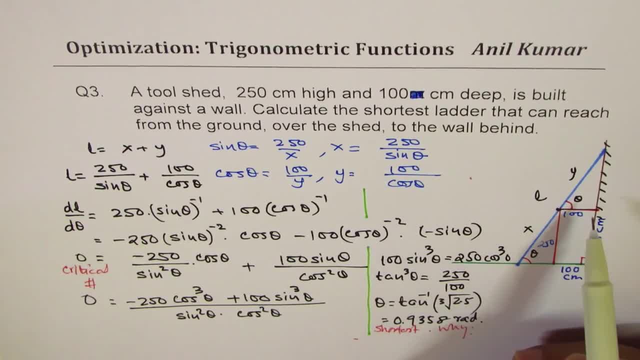 can you tell me? so it is shorted because one, we have two different conditions, that is to say, we could have a vertical rod right, which will be infinitely long, correct, or we could have a horizontal, which will be infinitely long. so, whatever is the answer, is the shortest that? 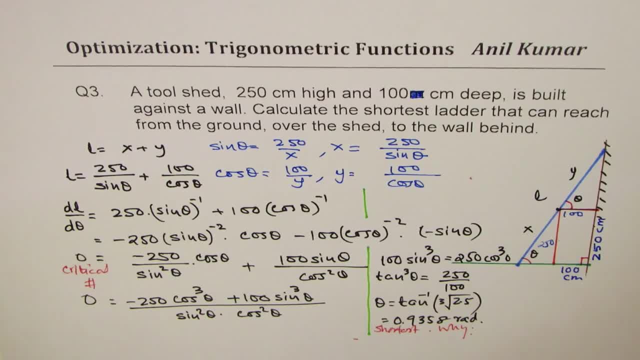 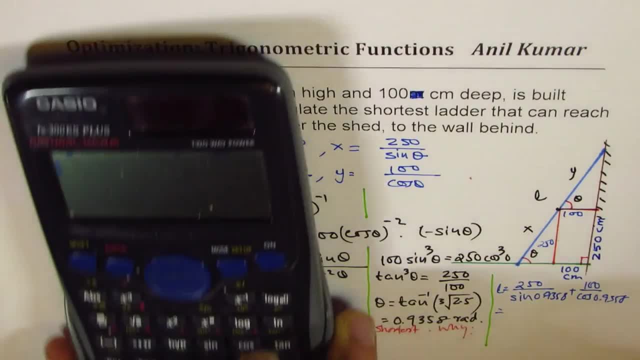 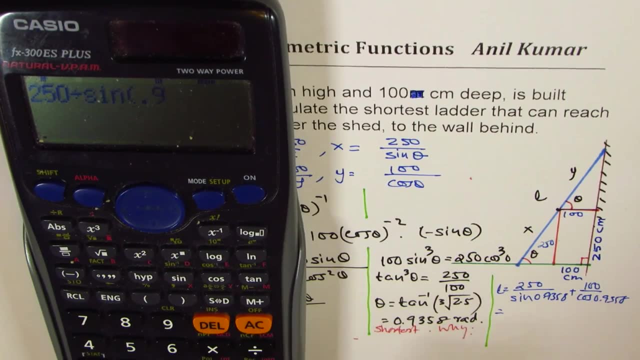 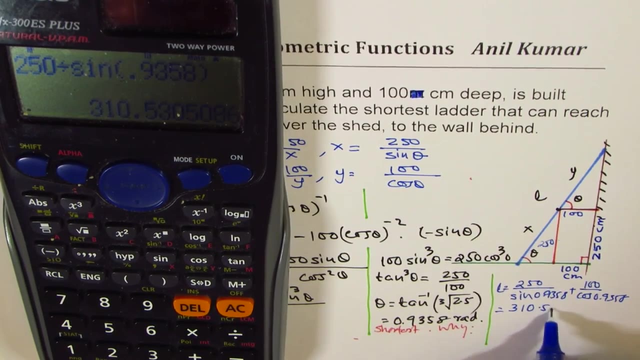 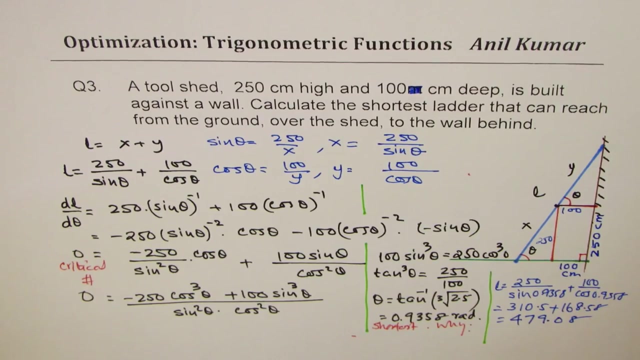 unreal grid. so that is equal to two fifty divided by sine point. 0.9358 equals to 310.5, plus 100 divided by cos of 0.9358, which is 168.58. let's add them 310.5, so we could write this as 479.08. okay, so around 479 centimeters is okay. so we get our.